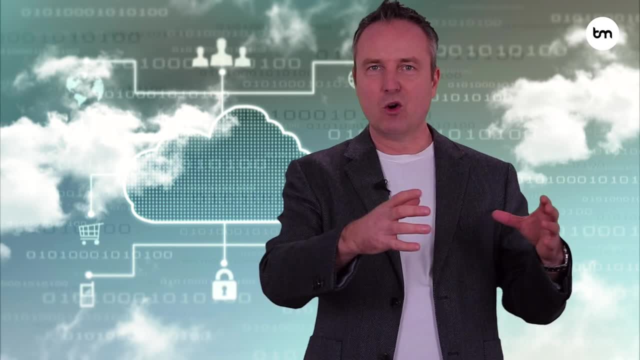 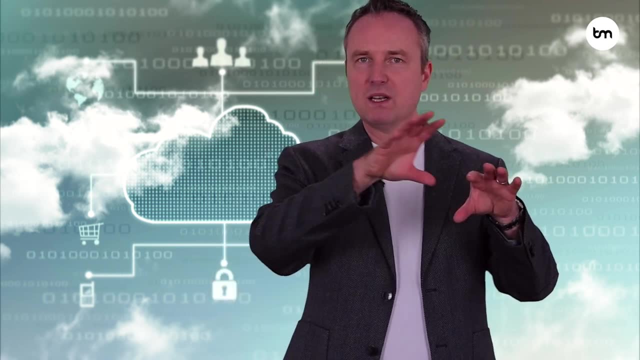 specific way. Google basically wanted us to search the internet in a specific way. Google basically wanted us to search the internet in a specific way- split second. They couldn't store the entire internet on a disk and then find the relevant information, So what they have come up with is storing bits of the. 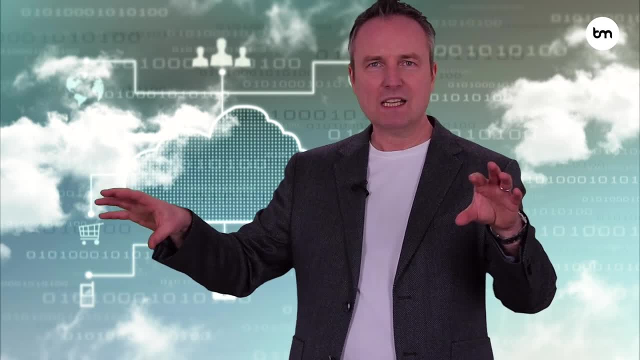 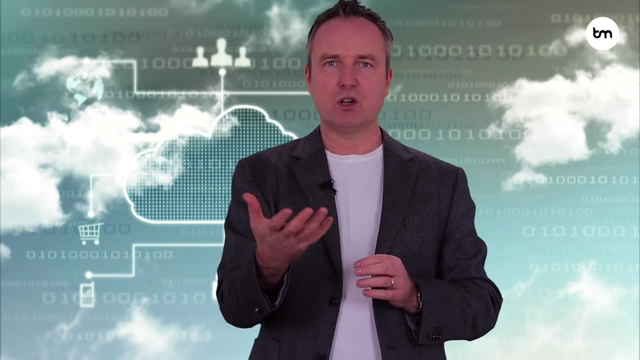 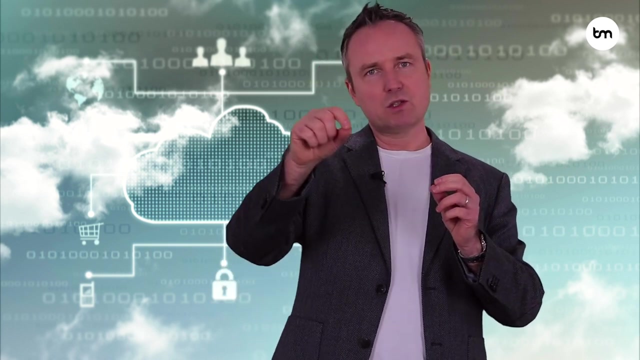 internet on computers anywhere in the world and then having these connected by the internet. you then break the analysis up. So if someone wanted to search for the internet or a specific bit of information on the internet, Google's intelligent software would then know where the data sits. it would break up. 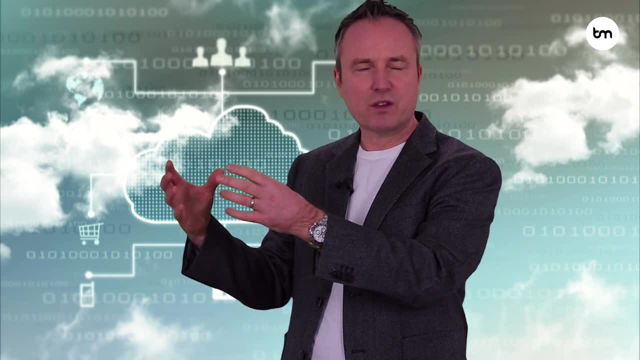 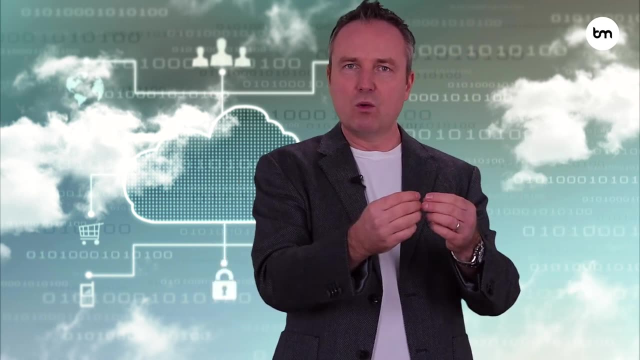 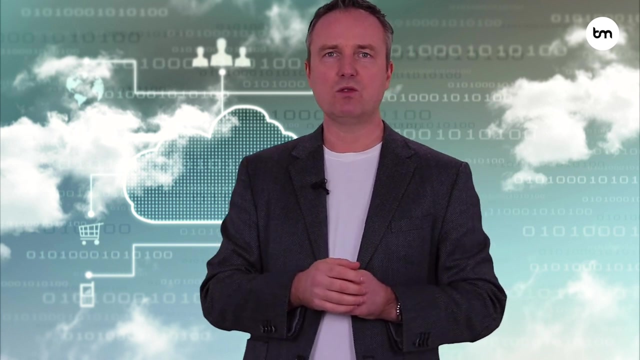 the analysis or use little servers, sometimes hundreds of thousands of servers who would all perform a tiny fraction, but in parallel. This would then all be aggregated up and in a split second you can get the result. Nowadays we use cloud storage and cloud computing all the time, So if you 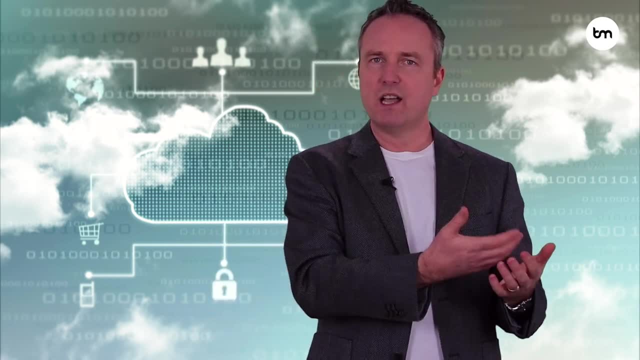 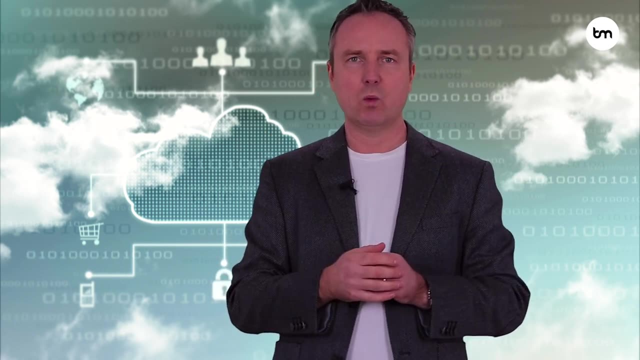 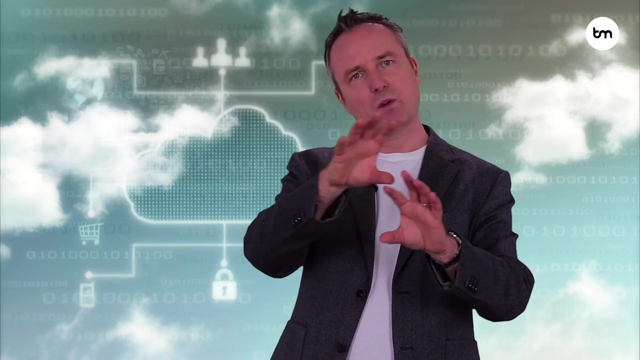 have an Apple phone, for example, you might use the iCloud cloud to store your photos, and this is exactly what we do. We store the photos on the cloud. We don't actually know where this cloud thing is, but it's probably a server. Quite often there's some redundancy, so we have 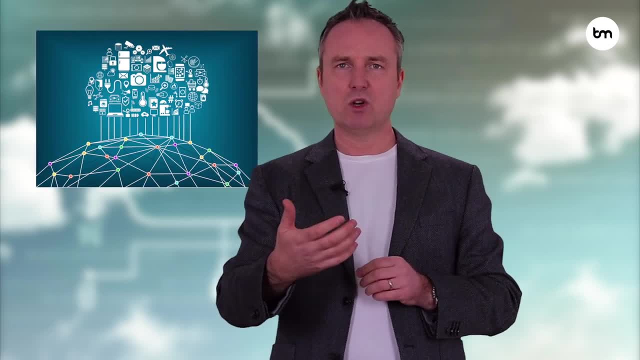 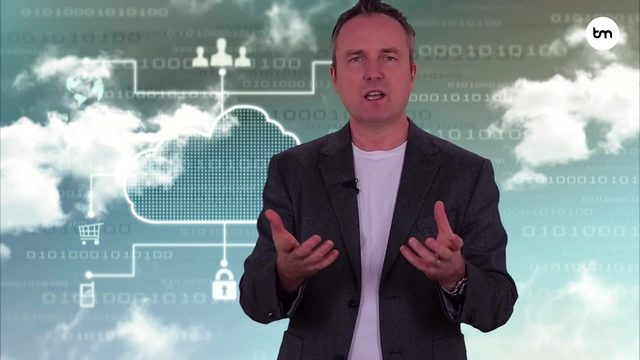 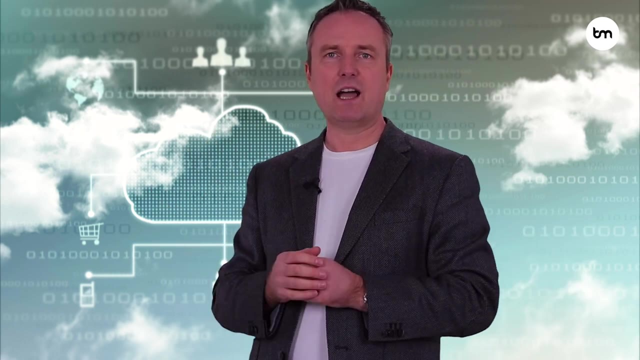 your photos on multiple servers across the world and if you want to look at it, it simply downloads it over the internet onto your device, And this is what companies now do Nowadays. it has broken down all the barriers to data storage and all the barriers to data analysis. So a company like Walmart, for example, 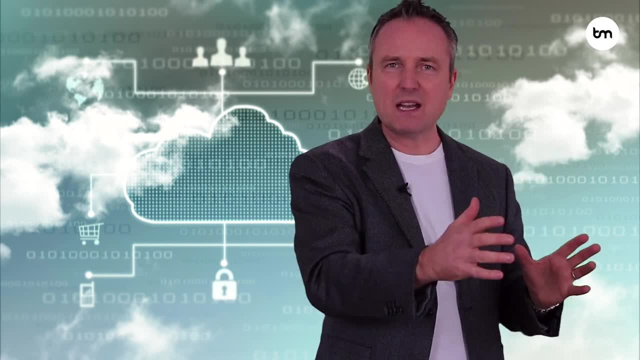 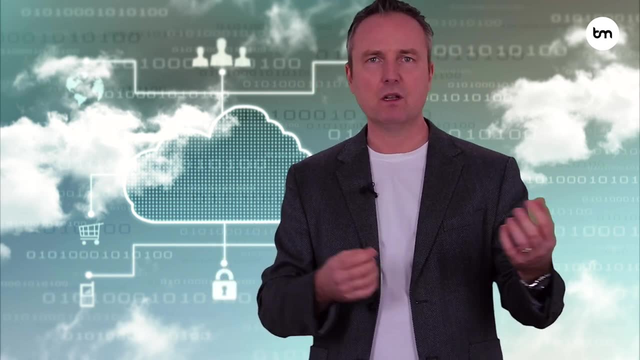 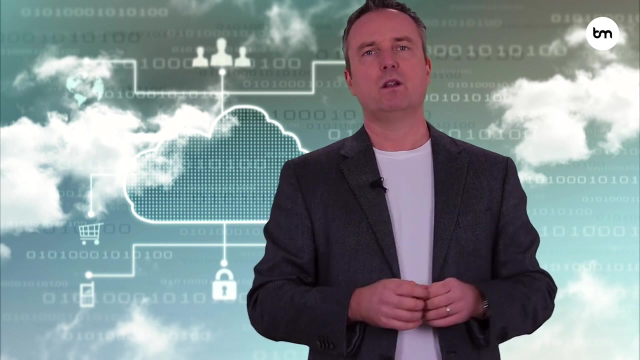 which generates two and a half petabytes of data every hour. they can simply go to companies like Microsoft or Amazon and say: please give me 150 petabytes of storage. They say, here you go, and then they stream their data to them. The other 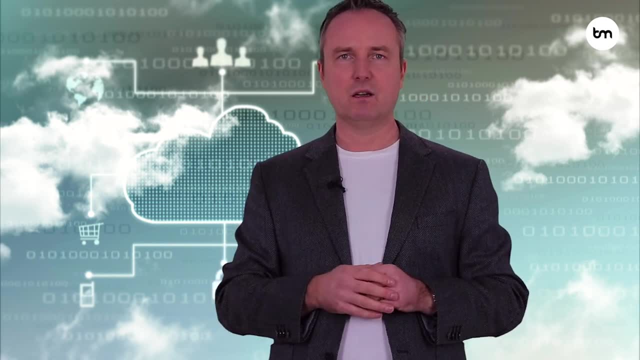 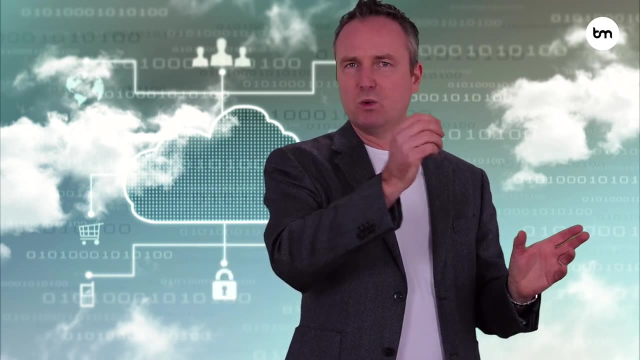 thing they do is they will give you the ability to analyze this data in almost real time, so we don't have the time lags. In the past, when you had huge data centers, sometimes you wanted to answer questions and these processors would crunch overnight and you come back and you get the answer. 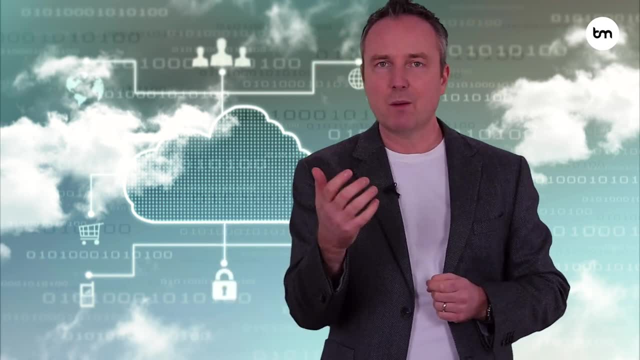 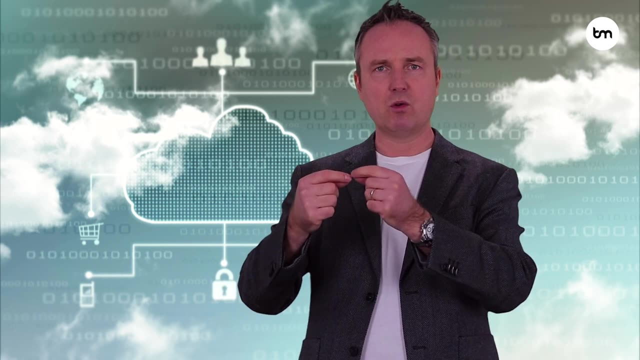 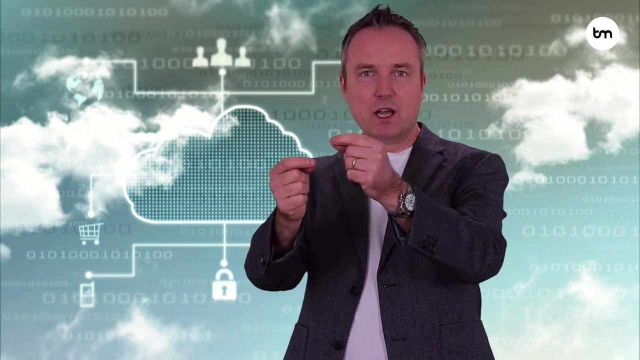 Nowadays, this is done in real time. so if you, for example, use your iPhone, you say, hey, Siri, where's the nearest Starbucks? What happens is that your phone records this. It then sends it via the internet to a cloud server. It will understand what you have said. It will then trigger a search on the internet to find 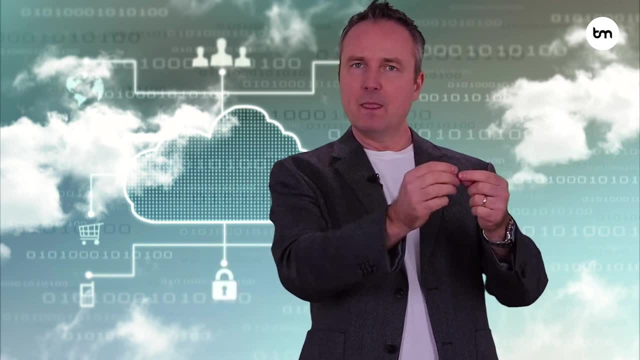 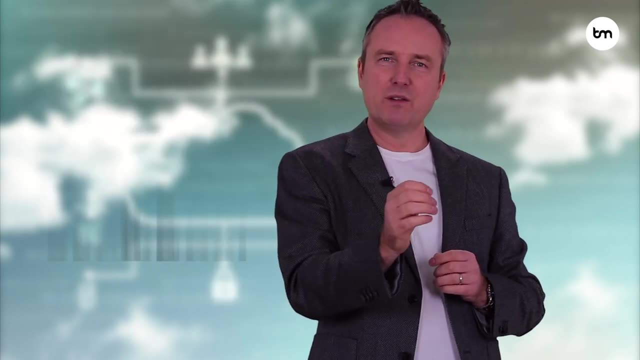 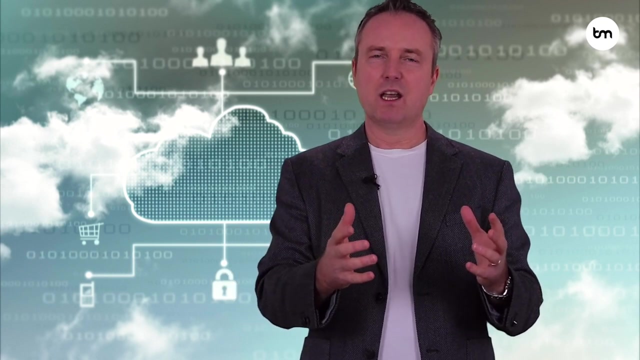 the nearest Starbucks using GPS information and other things, and then send the answer back to you. This involves over a hundred thousand computers, but takes 0.5 of a second. So this is what cloud computing is all about. It means any company can now store nearly unlimited amounts of data and 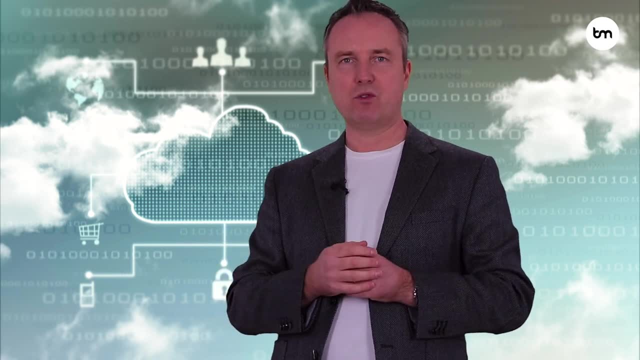 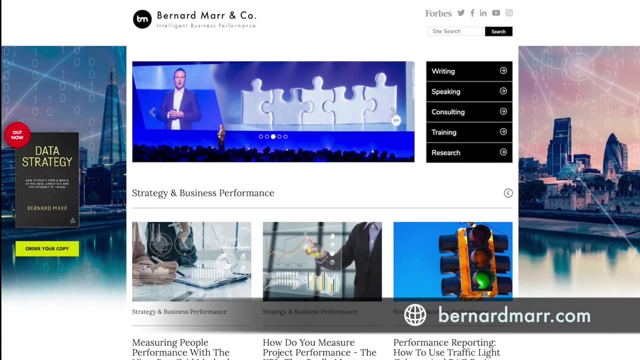 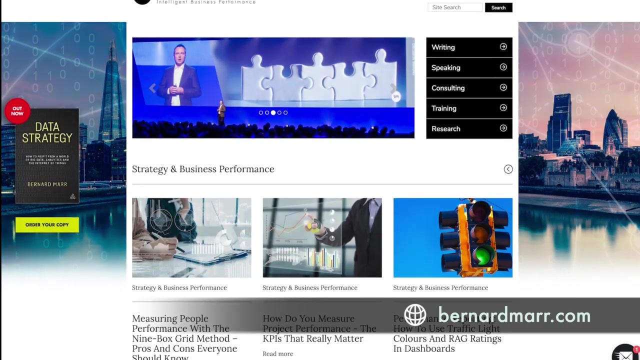 can analyze this data in real time To drive performance improvement. If you would like to learn more, head to my website at bernardmacom, where you can find tons of articles, white papers and videos that will give you a lot more insight into real-world case studies and.